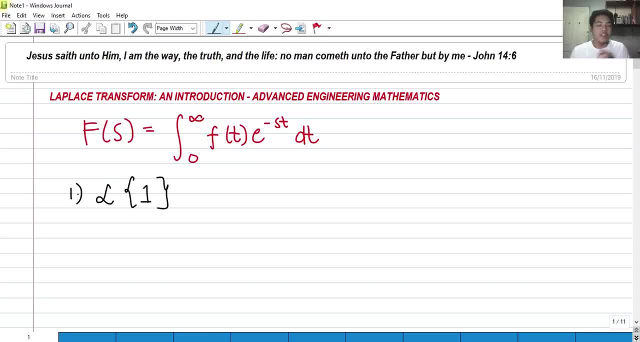 to s domain is the Laplace transform. So we shall be memorizing this formula in order for us to convert some function in terms of time into s domain. So let's get started For number one. what is the Laplace transform of the constant one? So here our f of t. 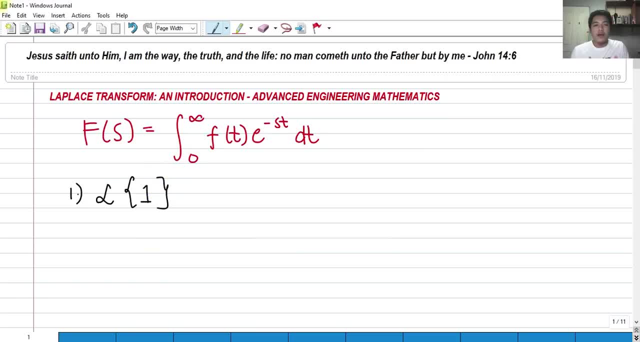 even though it has no term t included here, this is still considered as an f of t. okay, in time domain. So what is the Laplace transform? So simply we have. f of s is now equal from zero to infinity of f of t, which is one e raised to negative st dt. So simply. 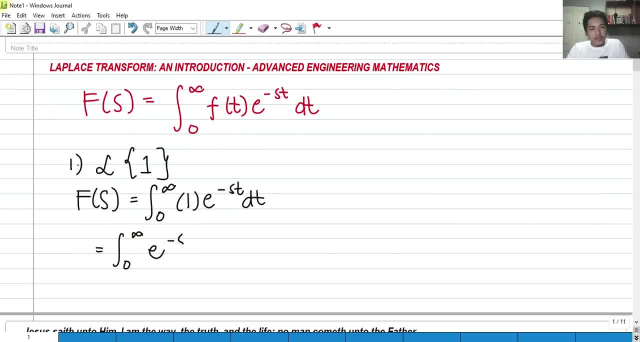 we evaluate the integral from zero to infinity of e raised to negative st dt. Okay, and remember that we are integrating in terms of t, So any other variable inside the integral is considered. any other variable other than t is considered as a constant inside the integral. So we have from zero to infinity of negative st dt. Okay, if we let, u is equal. 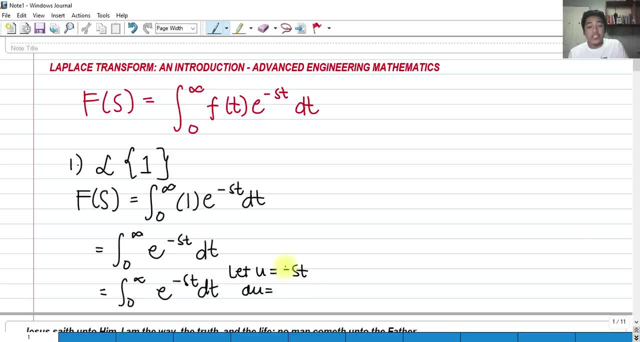 to negative st, our du is equivalent. With respect, we get the derivative of this. with respect to t is negative s dt. And if we get dt here, so we have dt is equivalent to du over negative s. So if we perform u substitution here, so we have. 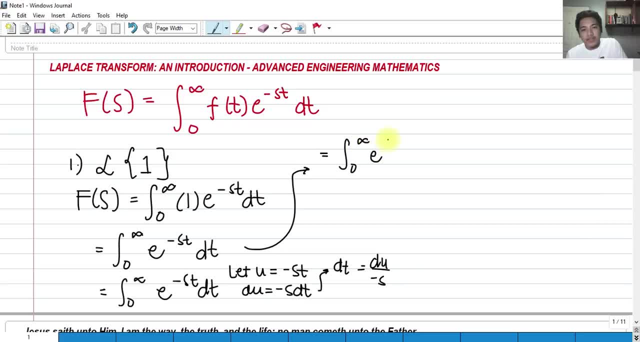 integral from zero to infinity. e raised to negative st, which is u. Okay, and our dt is du. over negative s. Okay, We have 1 over negative s because s is considered as constant here as we are integrating in terms of t, So we have negative 1 over s integral of from zero to infinity of e raised to u. 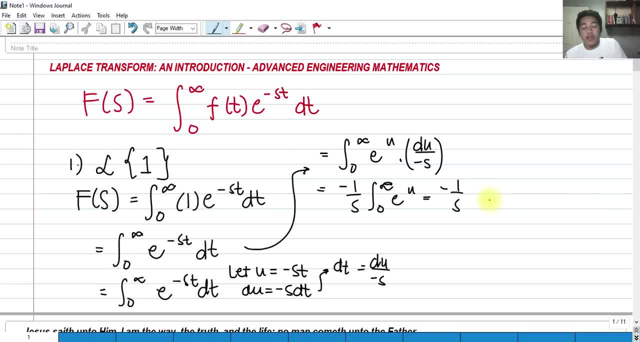 And we know that the integral of e raised to negative, e raised to u, is simply e raised to u. Okay, so evaluated from zero to infinity. So what will happen? We need to back substitute The value of u wherein u is equal to negative st. So this would become e raised to negative st. 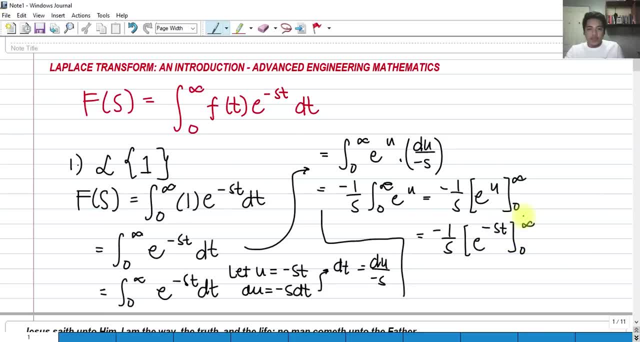 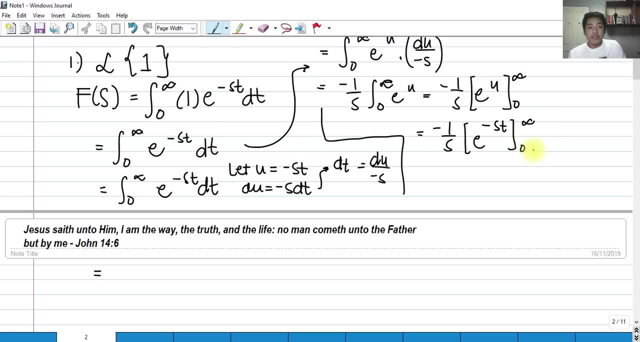 evaluated from zero to infinity. Okay, so we need to evaluate the definite integral or the limits. So we have negative 1 over st or negative 1 over s. e raised to negative s multiplied by the upper limit, which is the infinity minus. e raised to negative s multiplied by zero, the lower limit, So e. 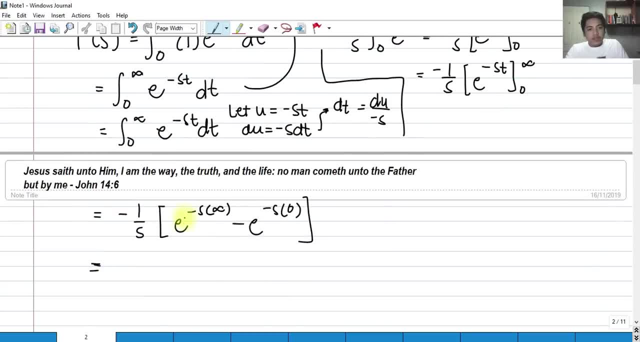 raised to negative s times infinity, This is considered as zero. This is equal to zero. 1 over s zero. So this is e raised to negative s times zero is e raised to zero that is equivalent to one. So if we multiply this, this is: this is 1 over st. 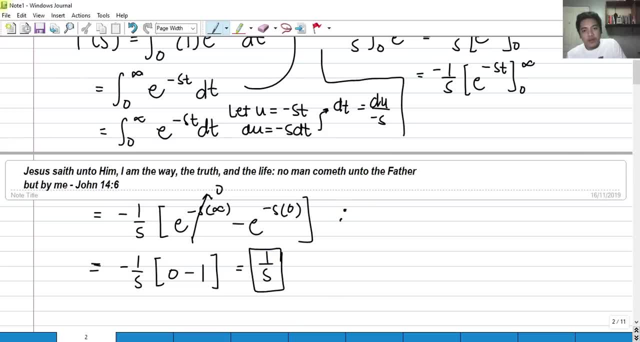 So the Laplace transform, therefore the Laplace transform of 1 is the f of s of 1- is simply equal to 1 over s. So that's the answer to our problem number 1.. The Laplace transform of a constant 1 is equivalent to 1 over s. 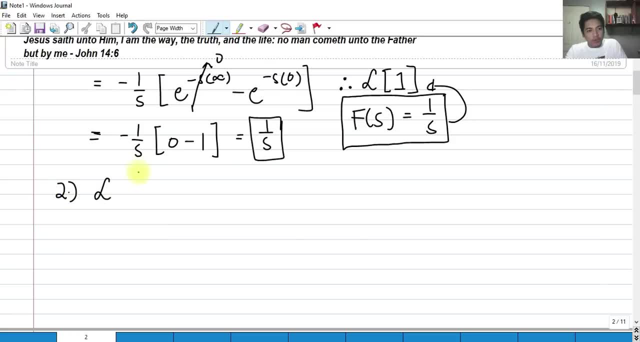 So let's try another one: The Laplace transform of a certain constant, let's say again 5.. So from the formula f of s is now equal to the integral, from 0 to infinity of f of t, e raised to negative st dt. 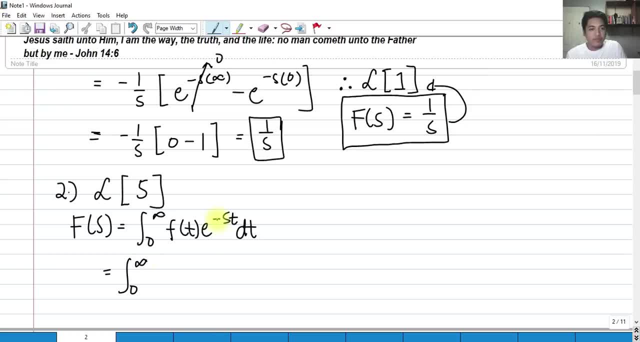 So we have from 0 to infinity, integral, from 0 to infinity of f, of t, which is 5, e raised to negative st dt, We can factor out 5.. Outside of the integral sign, So 5, integral from 0 to infinity, e raised to negative st dt. 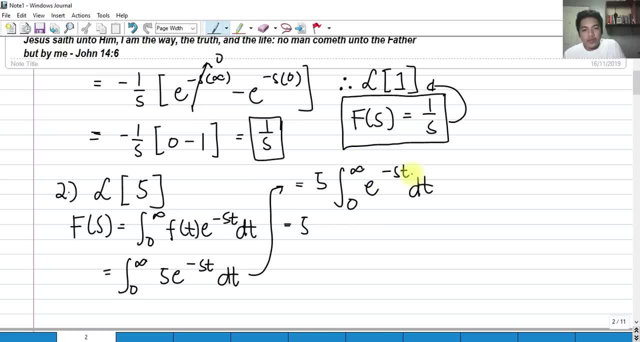 And we can again integrate this. If we integrate this again, we have to let. u is equal to negative st. Our du with respect to t is negative s dt, So our dt would now be du over negative s. So if we substitute that, we have e raised. 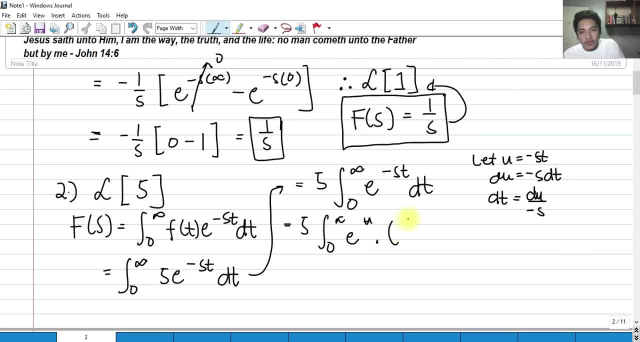 e raised to negative or e raised to u multiplied by du over negative s. Okay, So that is what dt is equal to. So I can factor out negative 1 over s, because we are integrating again in terms of u. So we have negative 5 over s here, from 0 to infinity of e raised to u du. 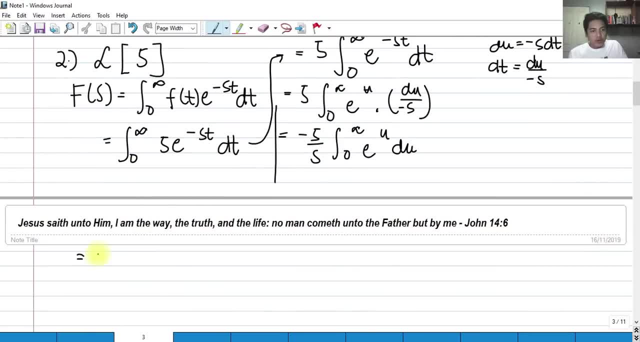 Okay, If we evaluate that again. So negative 5 over s. the integral of e raised to u is simply e raised to u, evaluated from 0 to infinity. Don't forget to back substitute what is the value of u. So we have negative 5 over s. 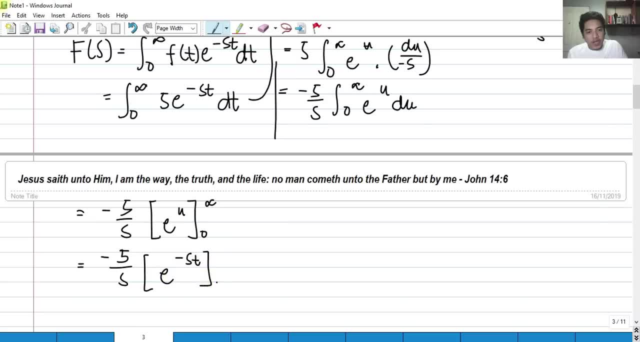 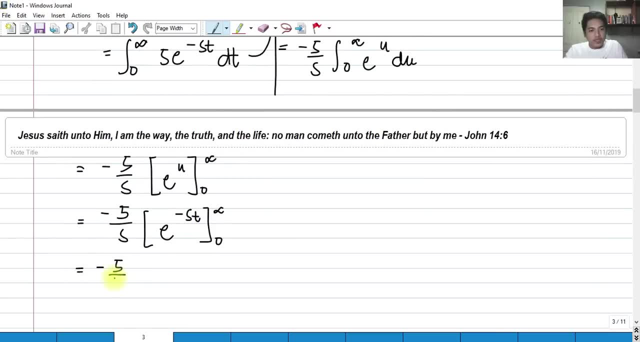 Okay, e raised to negative st. That's the original function or the original value of u. So what will happen here? Evaluating the limits? So we have e raised to negative s Multiplied by infinity minus, e raised to negative s multiplied by 0.. 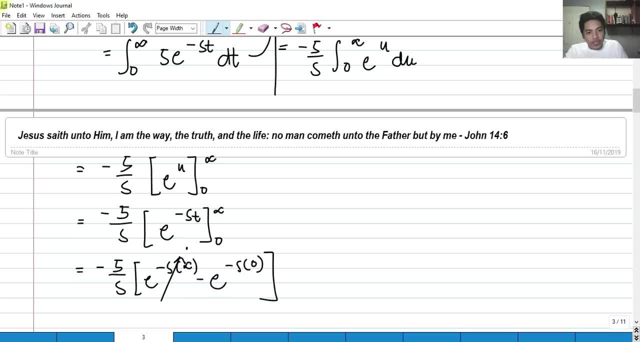 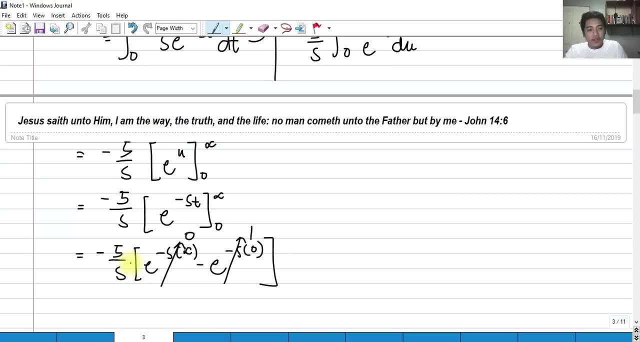 e raised to negative s multiplied by infinity is simply equal to 0.. e raised to negative s times 0.. This is e raised to 0, which happens to be equal to 1.. So what will happen? We have negative 5 over s multiplied by 0 minus 1.. 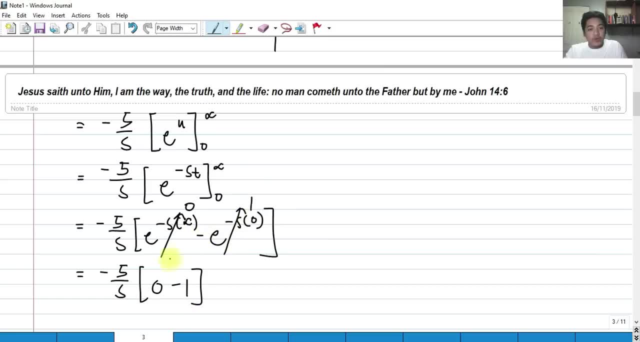 This is e raised to 0, which is 1.. We have a negative here, So we have negative 1.. So that is equivalent Equivalent to 5 over s. So simply, the Laplace transform of the constant 5 is 5 over s. 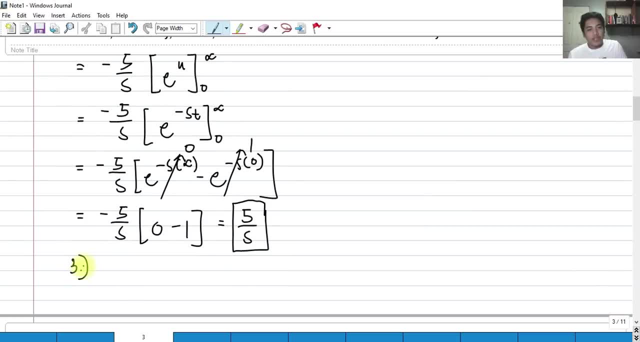 Okay, So the pattern here? Okay, Actually, we have a table If I'm going to get the Laplace transform of 10.. Okay, Simply, that is 10 over s. Okay, 10 over s, Because whatever the Laplace transform of a value of any constant, 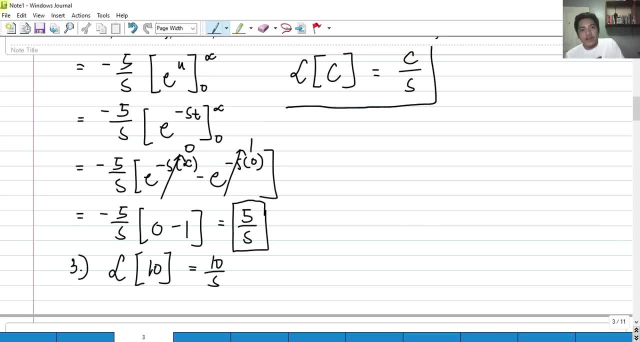 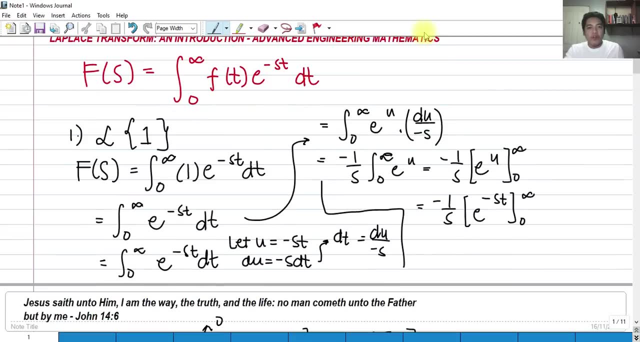 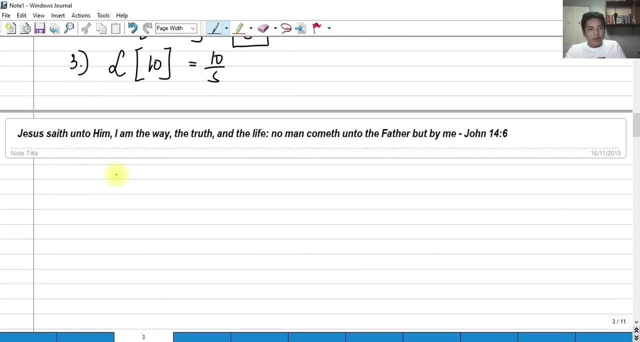 Is simply the value of constant over s. Okay, So I have shown you the hard way, Okay, The long method, Before we proceed to table method. Okay, So the table of Laplace transforms. So, for example, Let's say example number 4.. 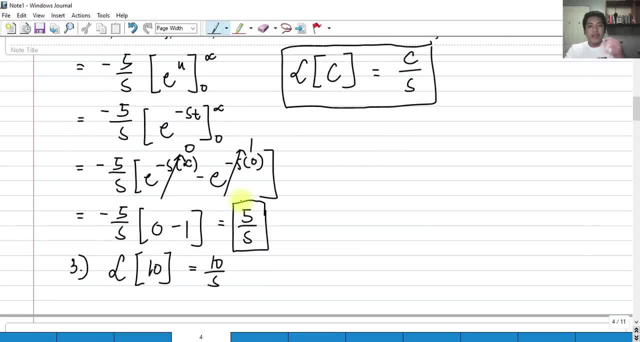 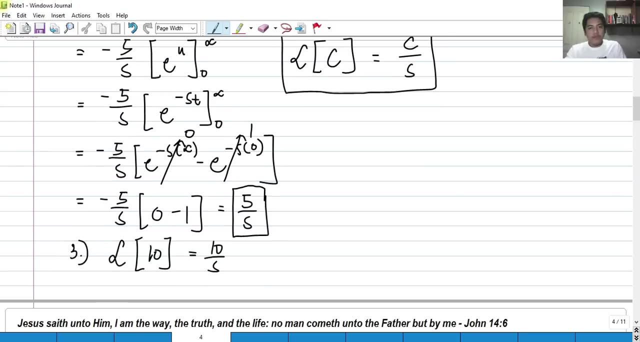 Okay. So simply again, If we get the Laplace transform of any constant, Okay, What will happen is The constant on the numerator divided by simply ds. Okay, So how about If we get, For example, The simplest f of t? 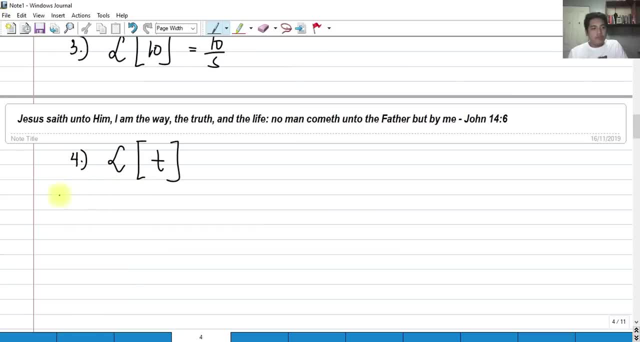 Which is t. Okay, The Laplace transform of t- Again we're going back to our formula- f of s Is now equal to the integral from 0 to infinity of f of t. e raised to negative st, dt Our f of t here. 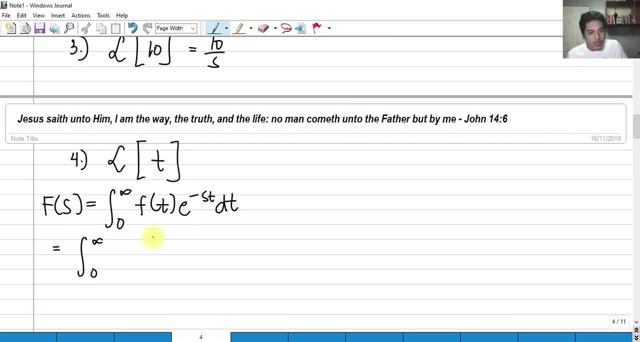 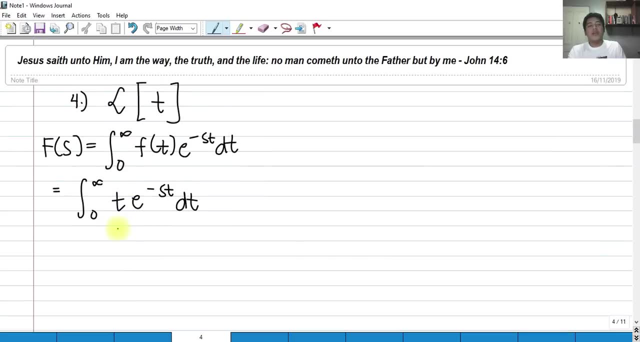 Is simply t, So we have 0 to infinity t Multiplied by e, raised to negative st, dt. So in order for us to get this, To get the integral of this, We need to recall Our integration by parts. This should be integration by parts. 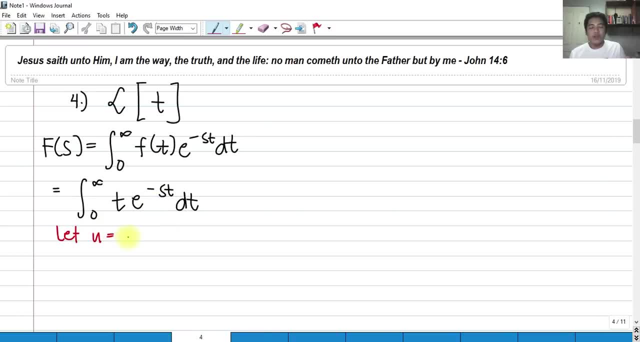 We have to let u. Priority in choosing u is liate Logarithmic, inverse, algebraic, Trigonometric and exponential Priority in choosing u. So this is What A polynomial Let's say With a degree of 1.. 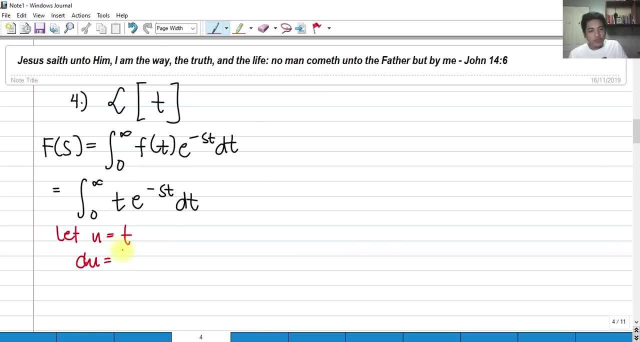 That is Let. u is equal to t, So the derivative of u with respect to t is simply dt. Okay, And the remaining Is our dv e raised to negative st dt If we integrate this to get v. Okay. 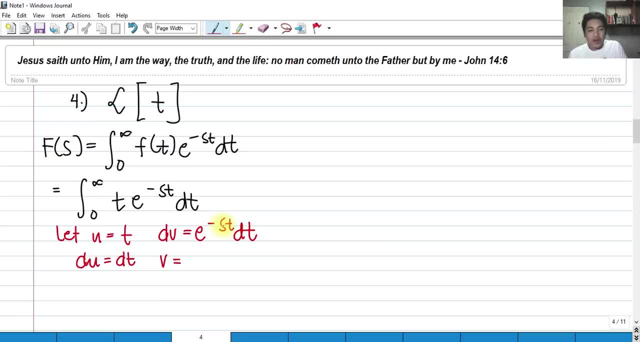 This is with respect to t, So any other variable is considered as constant. So what will happen? Use substitution again. We shall get Negative 1 over s e raised to negative st dt. Okay, If you are Confused. 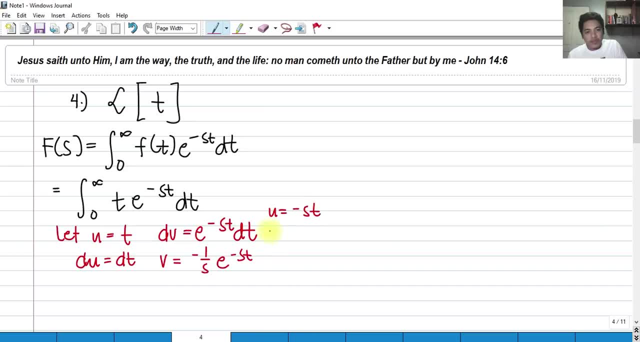 We. I choose u as Negative st again And du With respect to this Negative s, dt. And in terms of t? dt, I get dt. So that is du over negative s. So that's why we have a negative 1 over s here. 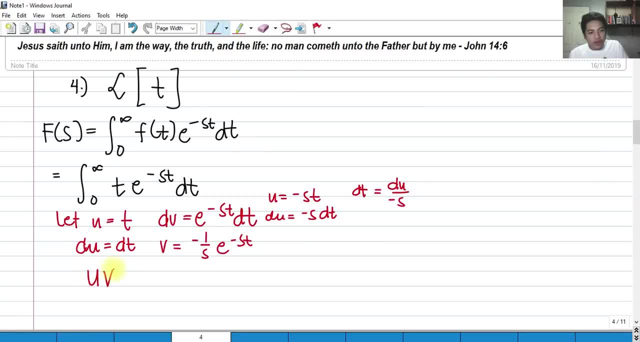 Okay, I hope that's clear, And we're going to use The formula By For integration by parts As uv Minus The integral of vdu. So what will happen? We have the integral. Okay, Let me just rewrite this here. 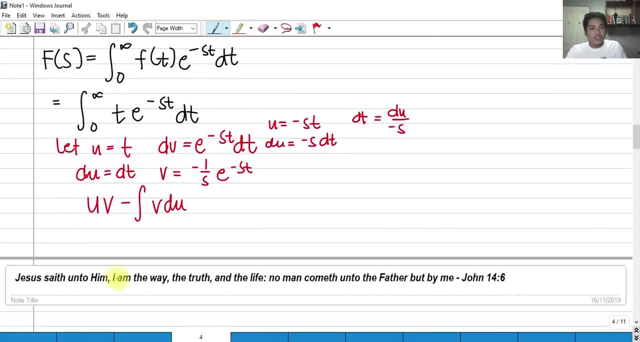 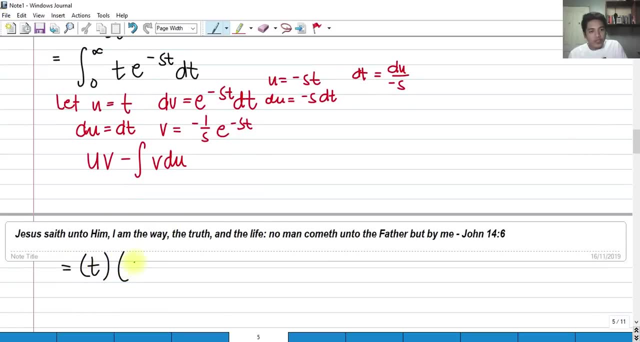 So we have the integral u, Which is t, Multiplied by v, Which is negative, 1 over s, e raised to negative st. Okay, Evaluated from 0.. To infinity: Okay, Because that's a definite integral, So we need to evaluate also. 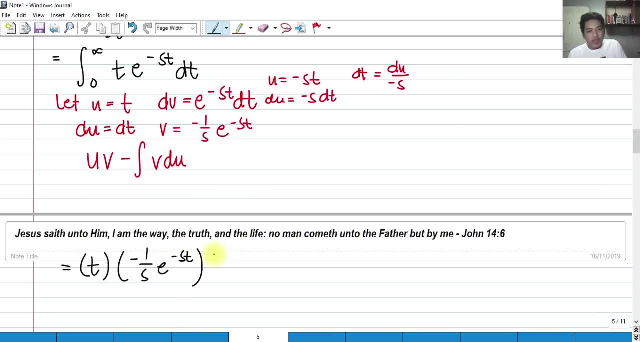 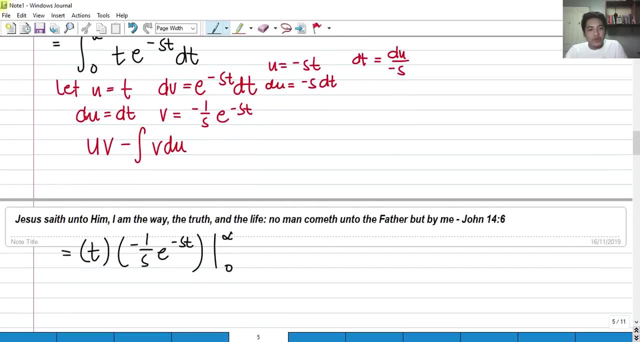 We need to distribute, Or The limits, So Minus The integral Of vdu. So what will happen? We have the integral. Okay, Let me just rewrite this here. So we have the integral u Minus. 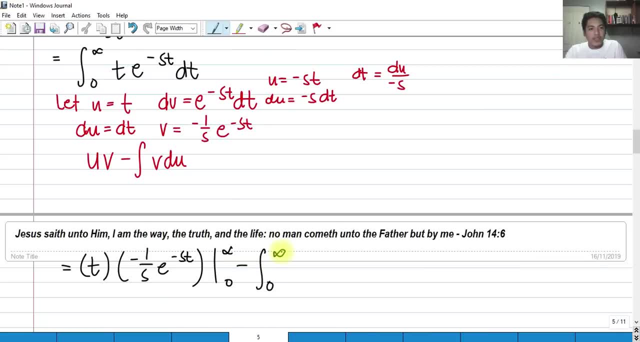 The integral From 0.. To infinity Of vdu. Our v Is Negative. 1 over s e raised to negative st. That is our v. Our du Is simply Equal to dt. Okay, So. 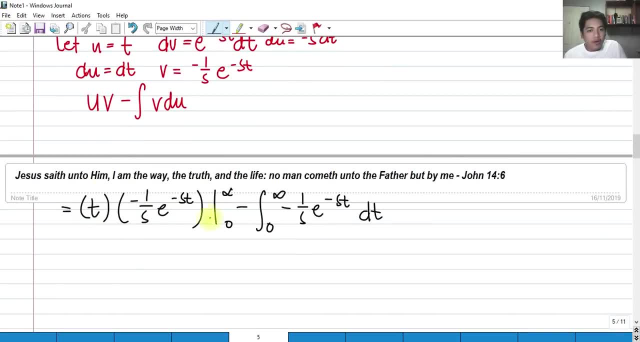 Let's first Evaluate The integral, Or Evaluate the limits here On the left side of our equation Or In this Side of our Term. So we have Negative t over s e raised to negative st, Evaluated from 0.. 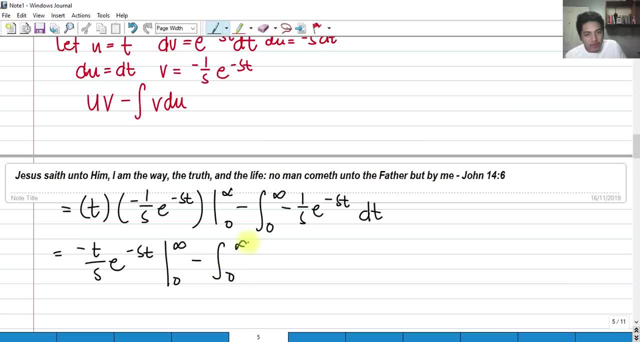 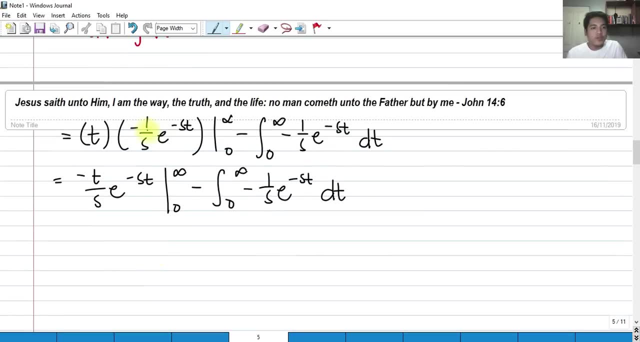 To infinity Minus The integral Of 0.. To infinity Of negative 1 over s e raised to negative st dt. Okay, So If I'm going to substitute Infinity And 0.. As the 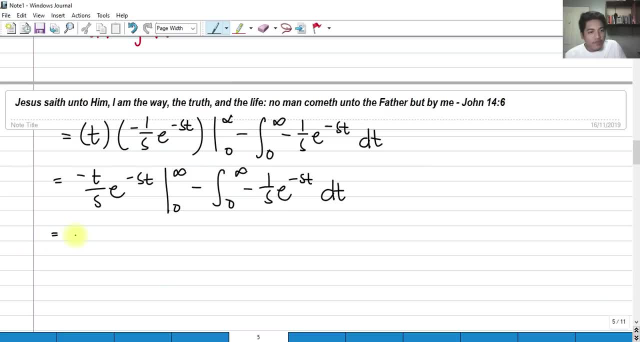 Higher And lower Limits In this Term. So we have Negative Infinity Over s. e raised to negative s Raised Multiplied By infinity. We know that. e raised to negative s Multiplied By infinity. 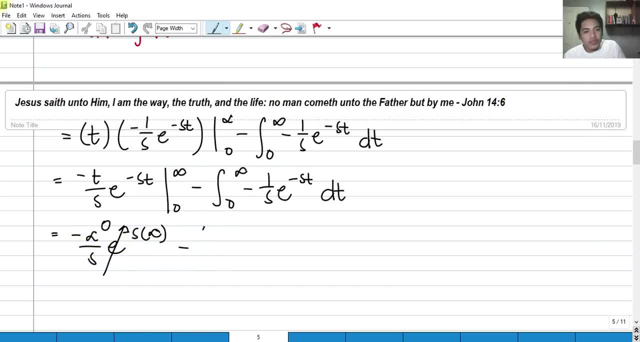 Okay, Because this is 0.. 0 multiplied by this Is simply 0.. Minus, Because That's definite integral Negative 0. Over s Okay e raised to negative 0. Times 0. Okay. 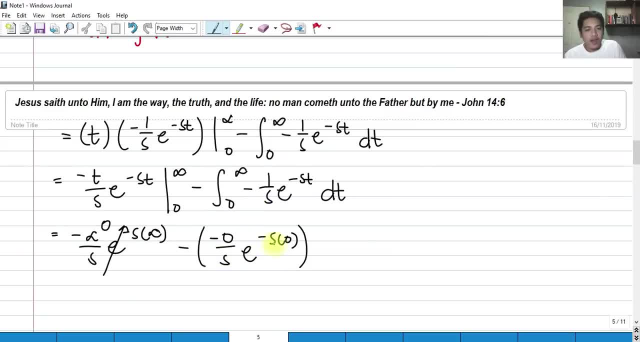 So 0. Over s, Simply 0.. If we multiply This By any Term here, So 0 times, Any number Would be 0.. Okay, That would be 0.. Okay, This is the minus. 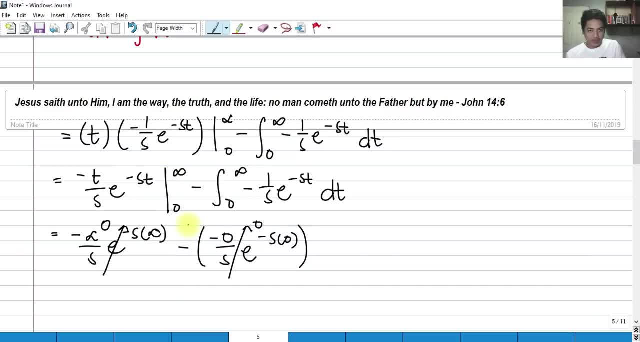 By evaluating the Definite integral. Okay, This is minus Because of this Again, And we have Again Minus Because of this. Okay, The integral From 0. To infinity Of negative 1. Over s. 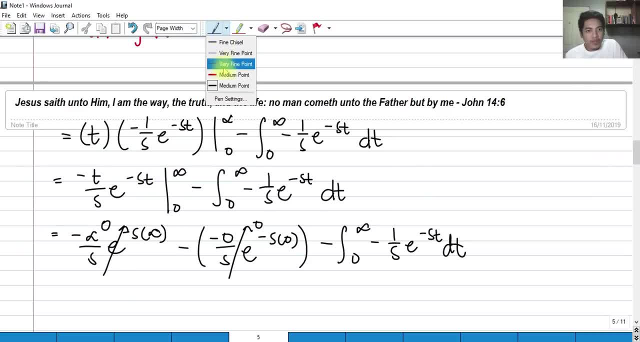 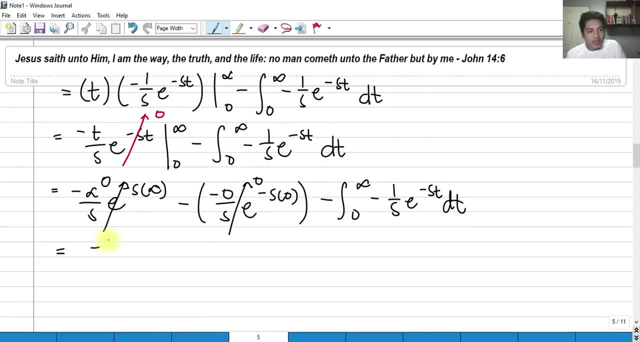 e raised to negative: s t Dt. So simply, This term Is equivalent Only to 0.. Okay, So Our Equation Simplifies This one Of The negative: 1. Over s e raised to negative. 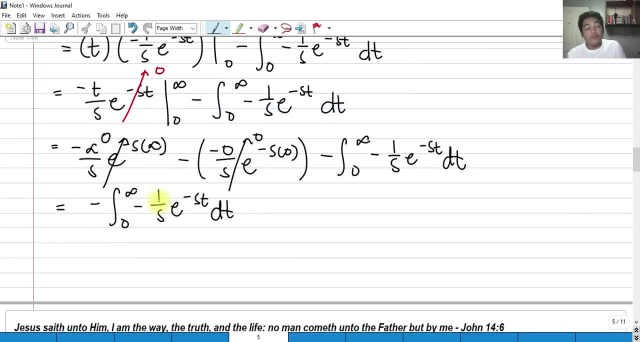 s t Dt Okay, So I can factor Out Negative 1. Over s Okay, Because We are integrating With respect To t And that is a constant, So Negative Times. 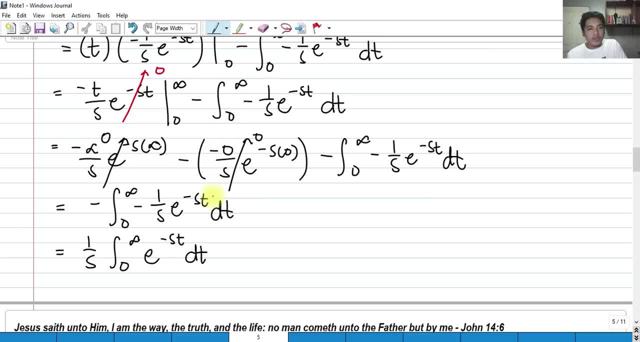 Negative: 1. Over s? t And in order For us To Integrate This, We have To Let Again: U Is Equal To Negative s t. Our Dt. 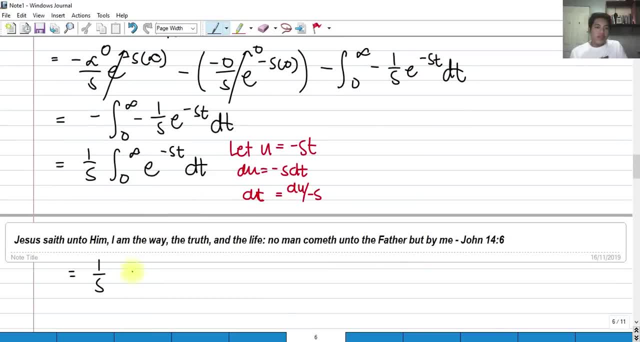 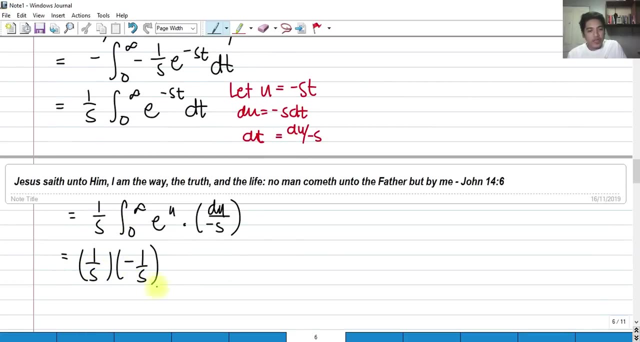 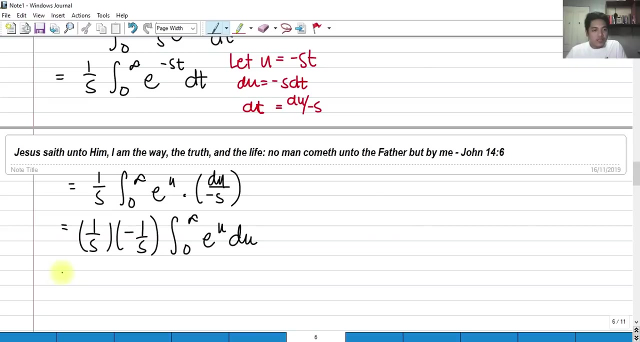 Therefore Is Du Over Negative S. So What Will Happen If I Can Factor Out Negative? 1. Over S Outside Of The Integral Sign. So 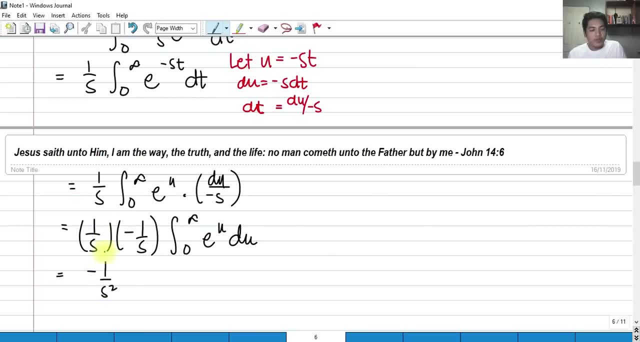 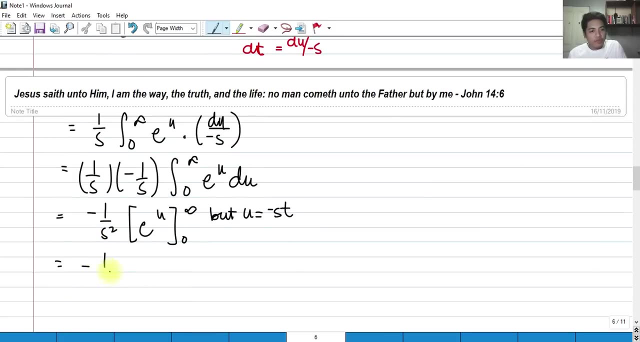 That Would Be 1. Over S Multiplied By Negative 1. Over S From 0. To S T. So Back Substituting That. So We 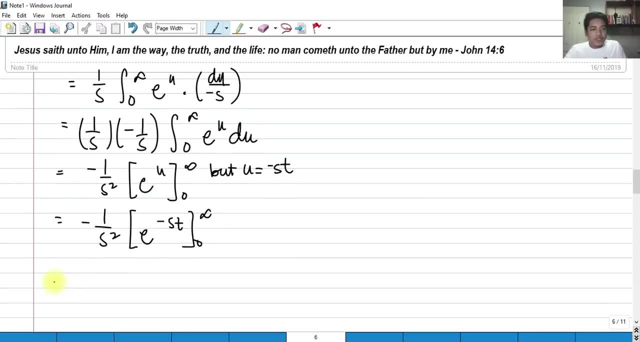 Have Negative 1. Over S Word Multiplied By E. Race To Negative S Multiplied By Infinity E Race To Negative 1.. So We Have. 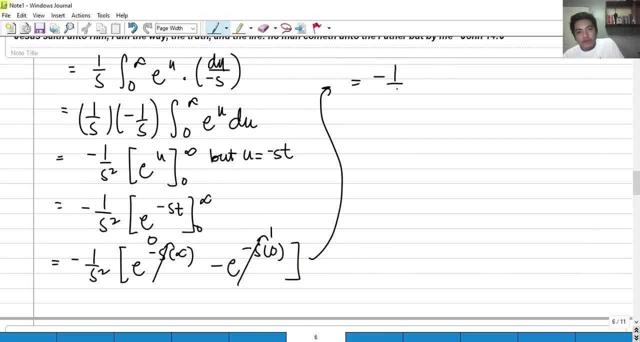 1. We Have Negative 1. Over S Squared Multiplied By 0. Minus 1. So, Or Simply Negative 1. Over S Squared. 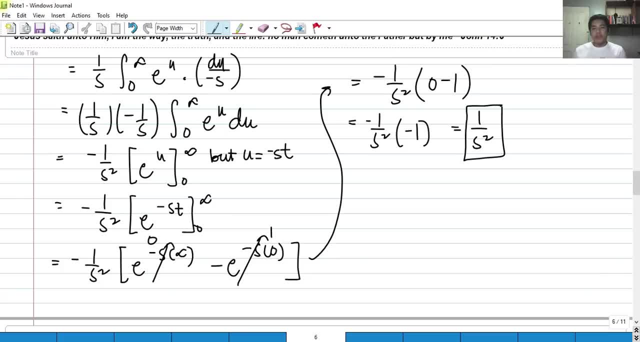 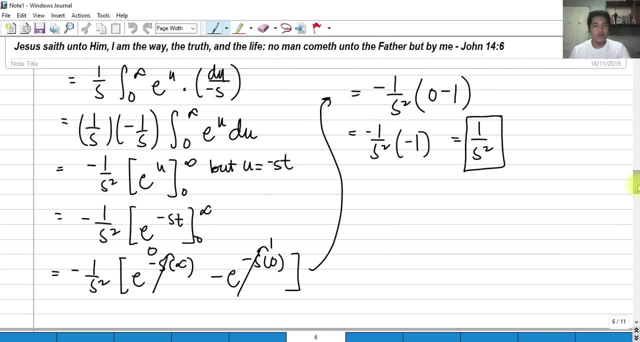 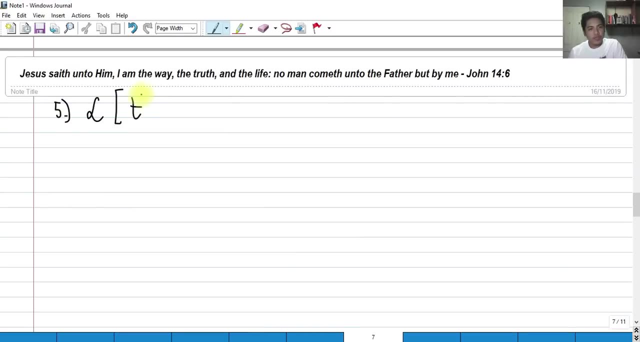 Multiplied By Negative 1. To 1. Over S Squared. Okay, So Let's Try To Solve Again Another Problem, Number 5. Let's Take 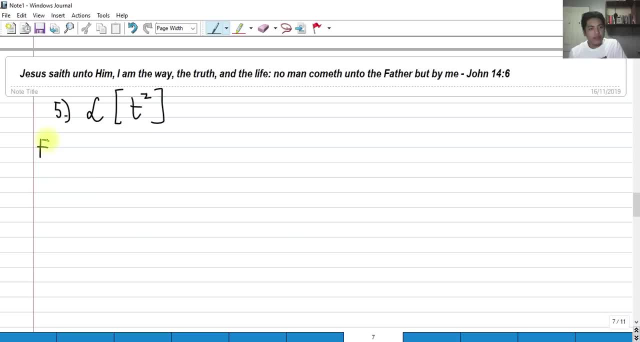 The Laplace Transform Of T Squared A While Ago. We Have T Multiplied By E Race To Negative S T D T. So Simply. 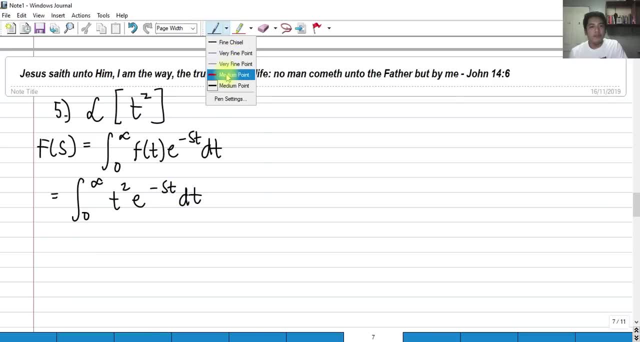 Substitute We Have, From 0. To Infinity Of The Integral Of T Squared Multiplied By E, Race To Negative S, T, D, T And. 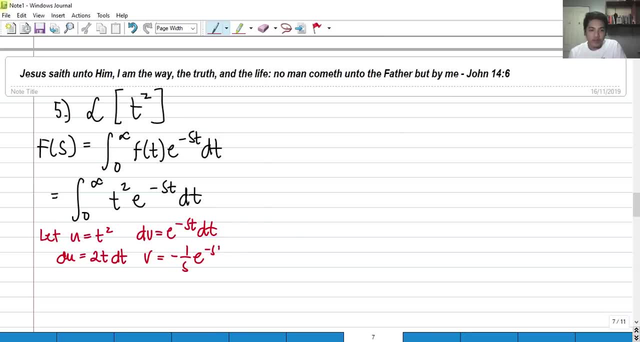 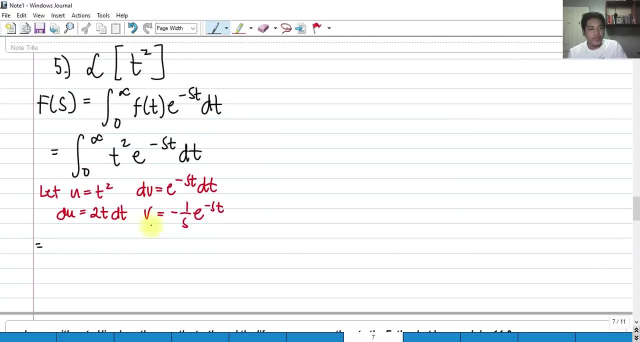 If We Integrate This Again. We Have Seen This A while Ago- That Is Negative. 1. Over S E Race To Negative S T Evaluated. 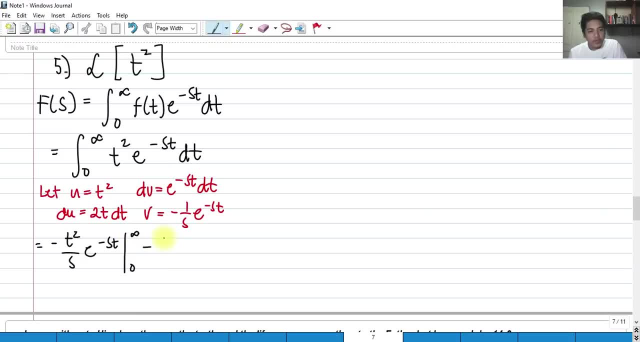 From 0. To Infinity Minus The Integral From 0. To Infinity Of V D U V D U, So We Have Negative 1. Over. 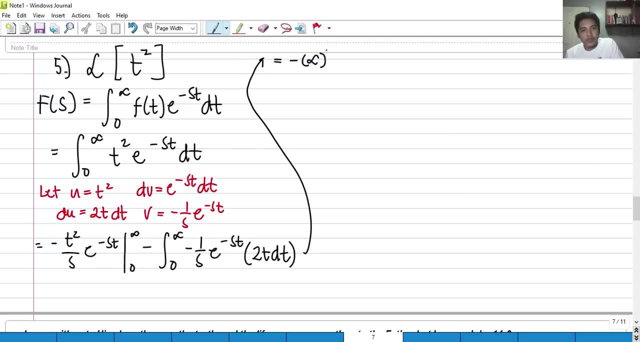 S E Race To Negative S Times, Infinity. Okay, Minus, That's Minus, Again Minus Because Of The Definitive Integral And We Have A 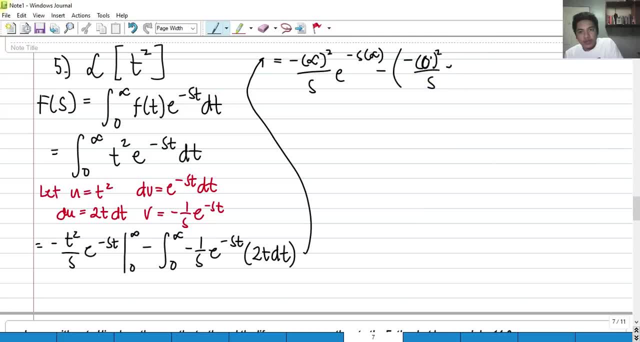 Negative Again Because Of This Function. The Original: Okay, This Is The That Minus Sign. That Is That Minus Sign I Can Factor Out To: 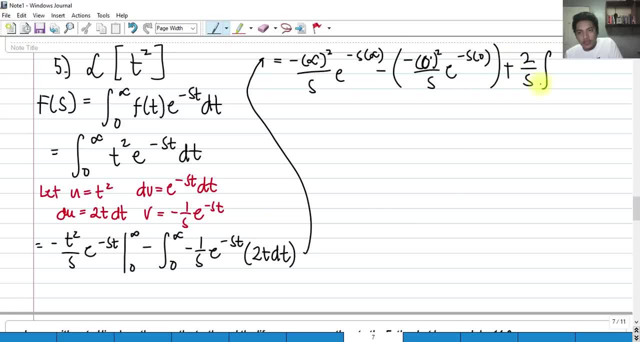 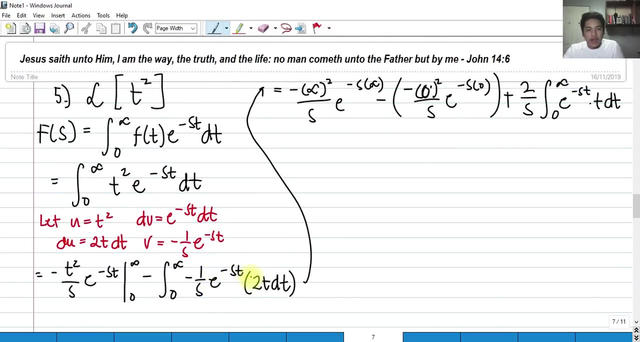 And Negative 1. Over S. So If I'm Going To Multiply To, Why Did I Choose? Okay, Why Did I Choose To Actually Factor Out? 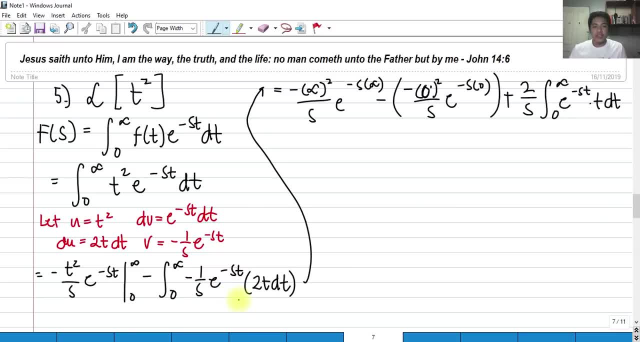 Negative: 1. Over S Outside The Integral, It's Because We Are Again Integrating With Respect To Zero And Again This Is Zero In The 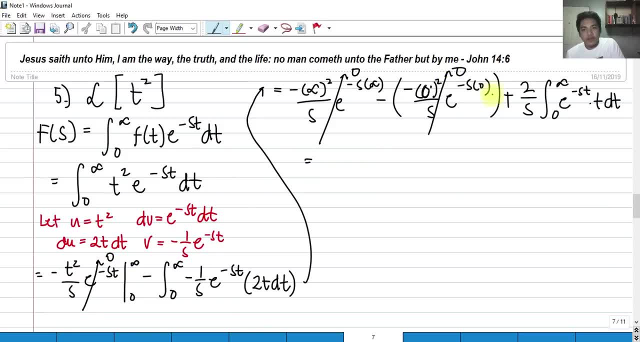 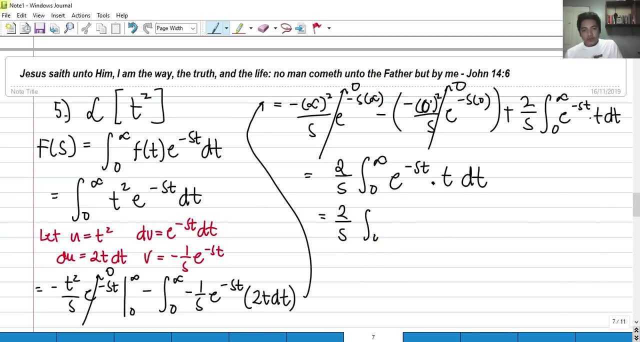 Denominator In The Numerator. So Zero Multiplied By Any Number Is Still Zero. So The Whole Term, This Whole Term Again. This Is An 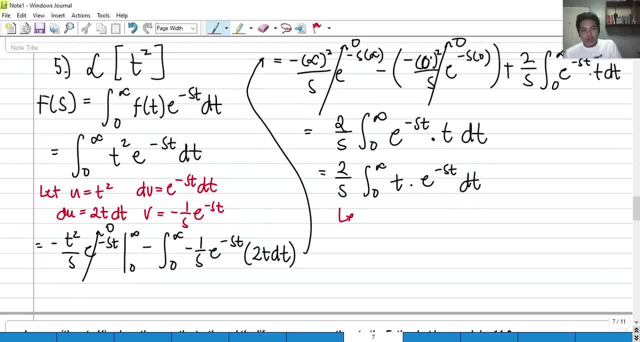 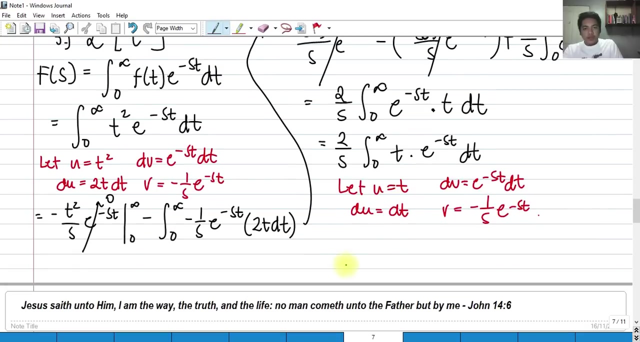 Integration By Parts Again. So We Have To Let You Equal To T Our D? U Is Equals To Simply D T Our D? V Again. 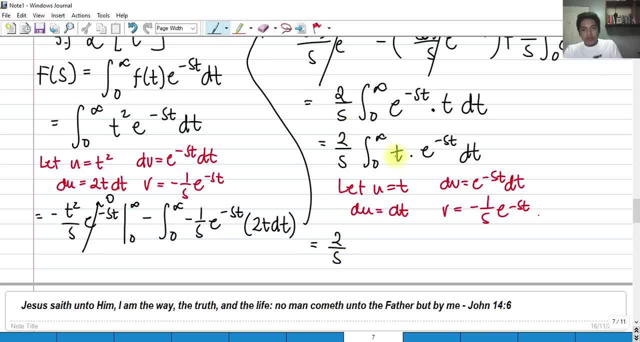 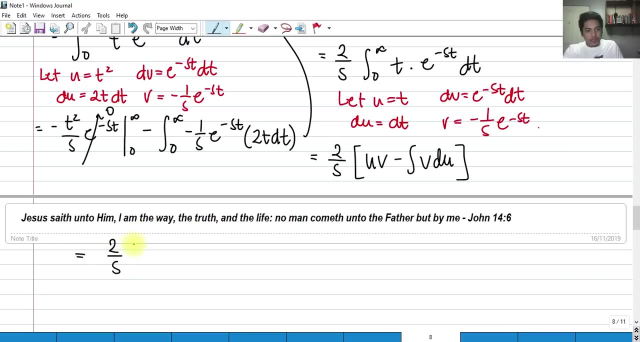 This Is Outside Of The Integral. So Whatever The Integral Of This, This Is Multiplied, So We Have U V Again Minus V D U. 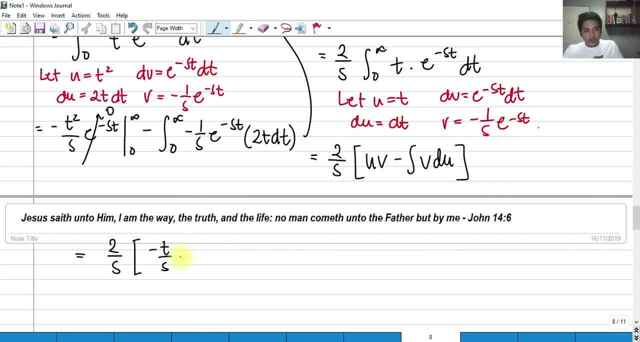 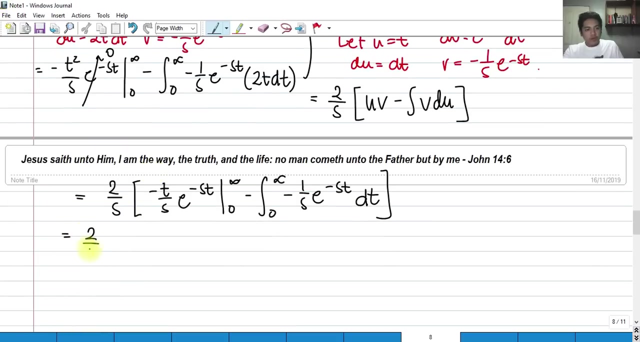 That's The Integral. For The Integral Of V D U. Negative One Over S? E Is Negative. S T Our D? U Is Simply Equal. 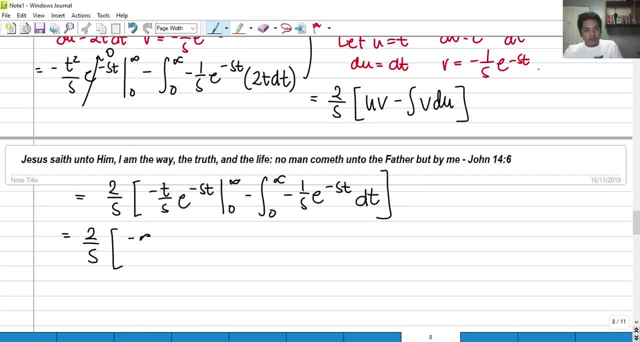 To D T. So Two Over S Multiplied By Minus Negative Zero Over S, E Is Negative S Times Zero. We Know That This Is. 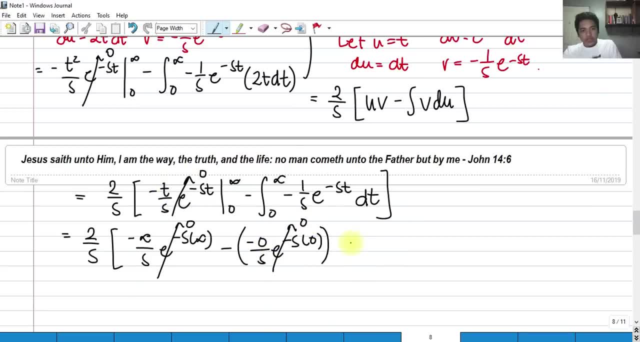 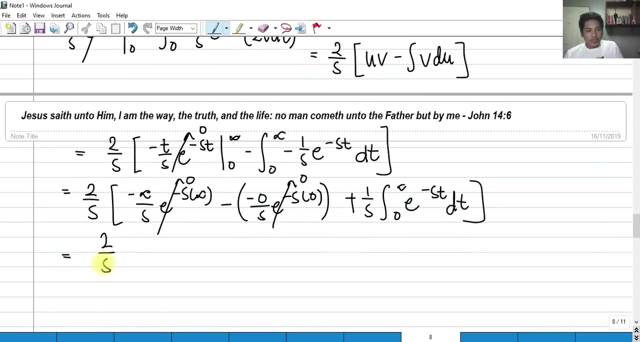 Also Equivalent To Zero. That's Right, Because Zero Times Any Number Zero, So This Will Become Plus One Over S Integral From Zero To Infinity. 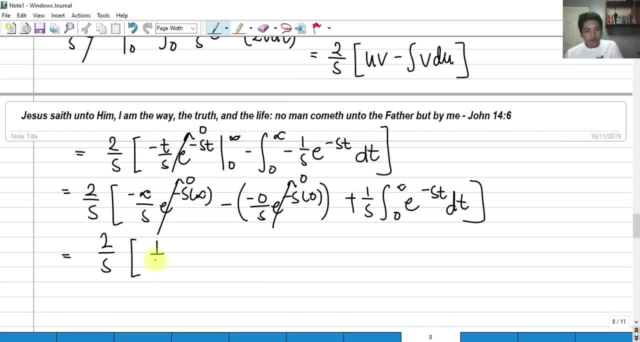 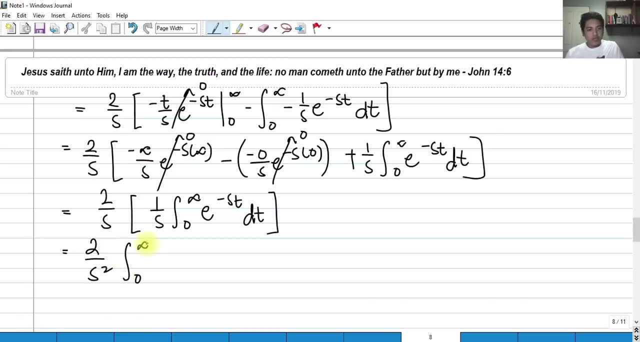 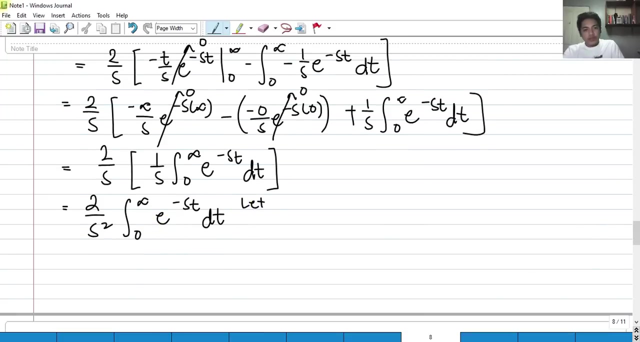 Of E Is Negative, S T, D, T. So Again, To Simplify, We Have Two Over S Integral From Zero To Infinity Of E Is 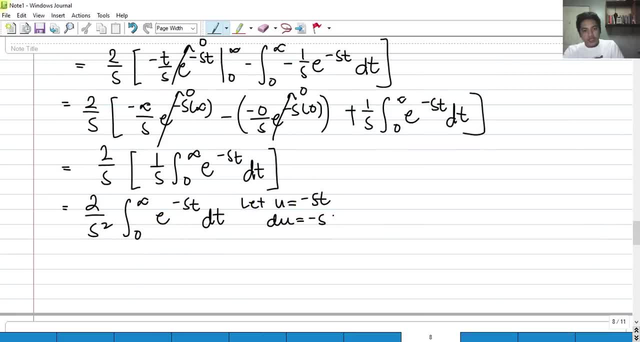 Negative S T D T, And The D? T Now Is Equal To D? U Over Negative S. So We Have D? U Which Is D. 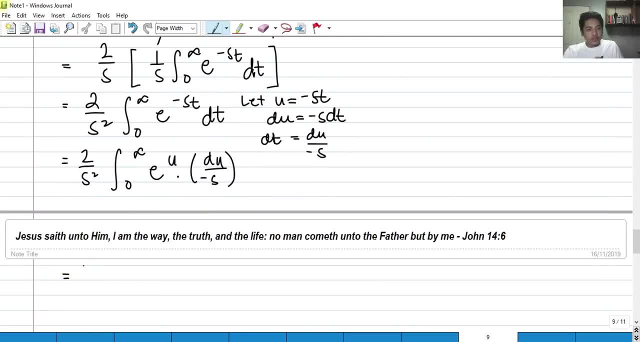 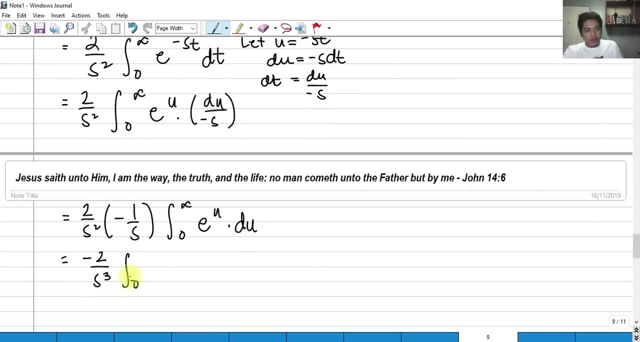 T, Which Is D? U Over Negative S I Can Again Factor Out Negative One Over S Outside Of The Integral S Integral From Zero To. 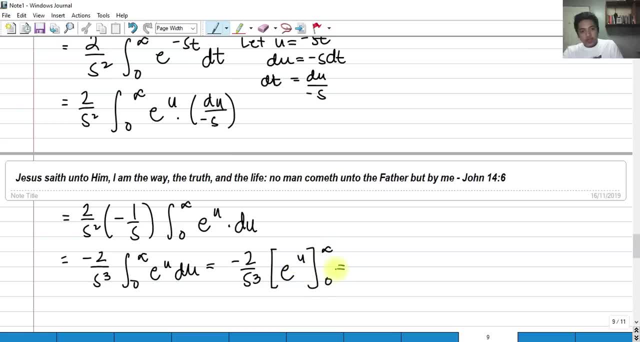 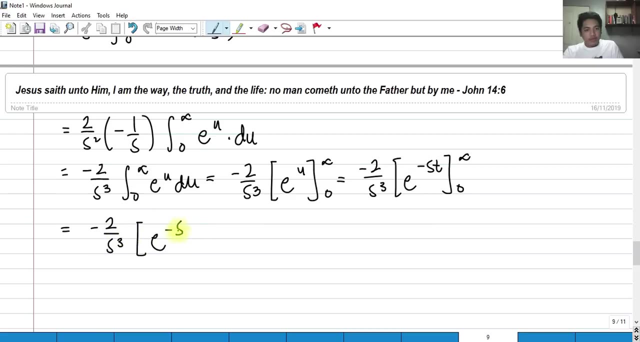 Infinity, But Our U Is Equivalent Again To Negative. S T Alright, So From Zero To Infinity. So, Evaluating The Limits, So We Have Negative. 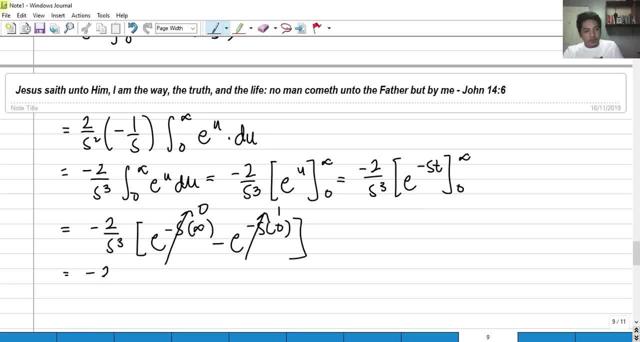 Two Over S Cube Multiplied By Zero Minus One, Or Simply Negative. Two Over S Cube Multiplied By Negative One Is Simply Two Over. 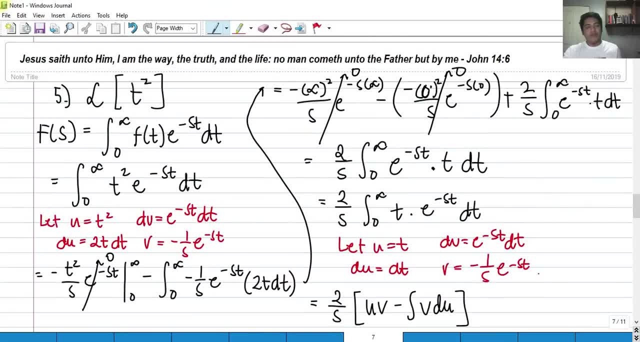 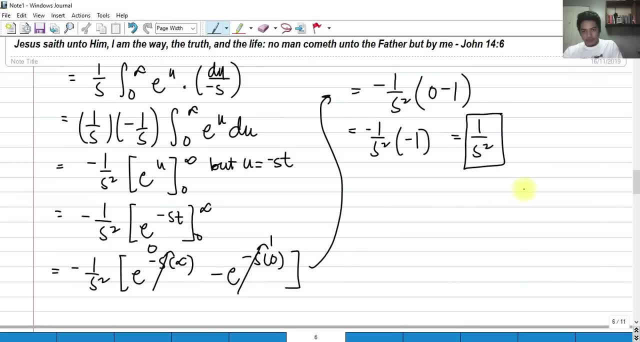 S Cube. So That Is The Plus: Here We Have A Formula In Actually Finding The Laplace Transform, Okay, Laplace Transform Of Any T Raised.